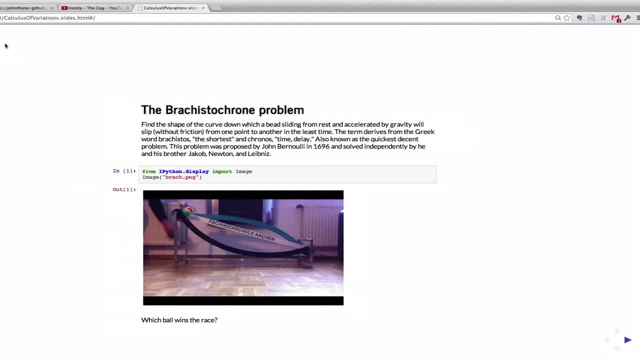 two points is a straight line, right? So why wouldn't number 2 win? Because it has to travel the shortest distance. So who says number 1?? Who says number 2?? Who says number 3?? 1, 2, 3. Number 1. Okay, 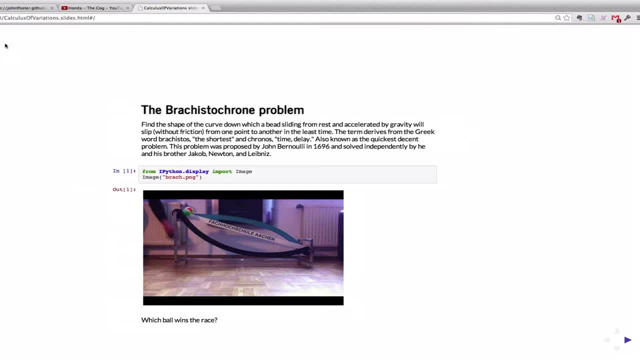 I got two answers. No one else is answering right? Okay, So we're engineers, Let's, let's, let's, let's not guess right, We're engineers, Let's, let's compute the solution. So the 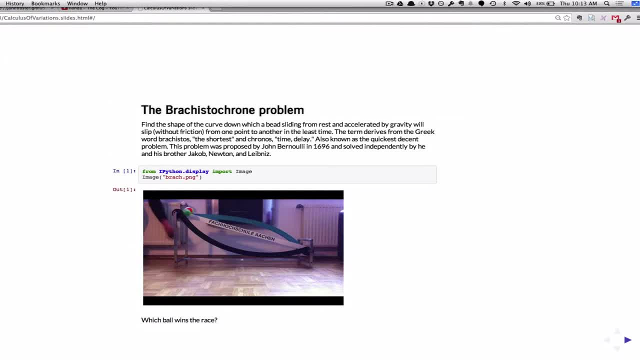 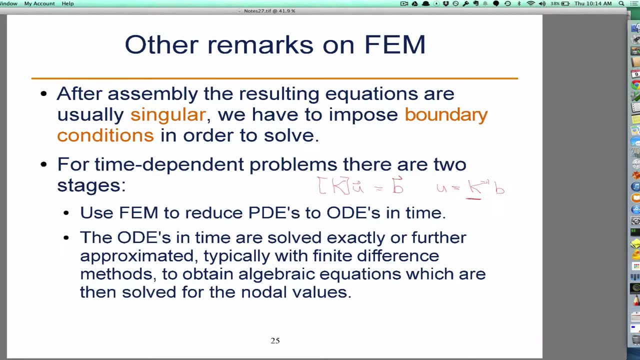 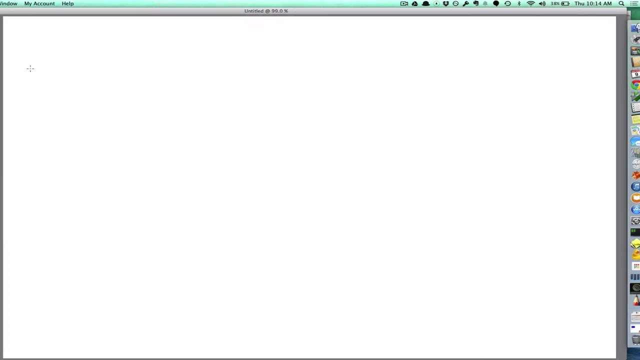 problem that we're faced with. The problem we're faced with is a famous problem called the Bacrytochrome problem. 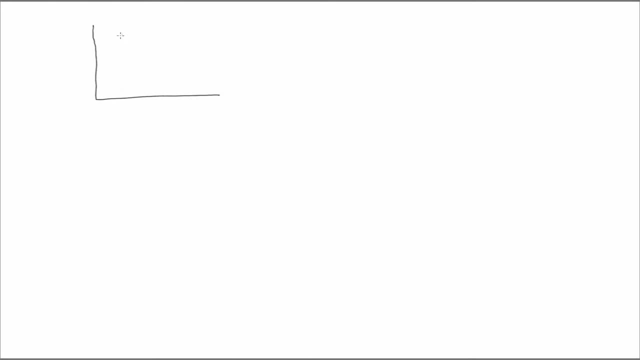 If we have two points and a particle that's going to travel along those points under the action of gravity, what is the fastest path between the two points, Meaning the fastest path in terms of time? So the question is: a particle traveling from point A to B, what is the path that will get you there the fastest? 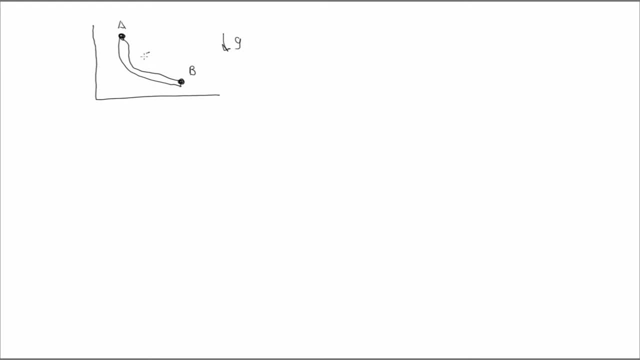 And so if we call our path S and we zoom in on a little increment of S dS, we can approximate dS as the square root of dx squared. Okay, And I'm going to write: well, basically, if you divide by dx, you can show that this results in 1 plus y prime. 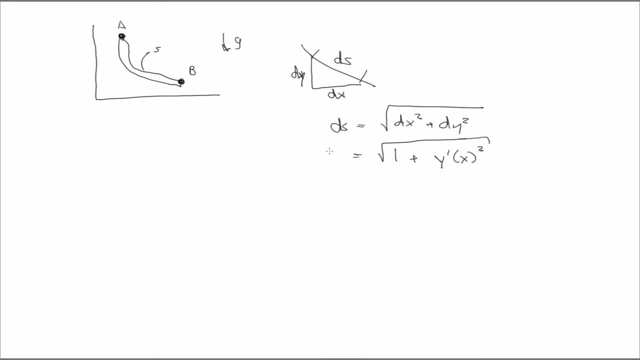 of x squared. Okay, And so the time? so that this is just an approximation to our path dS, And we can show that the time it takes is equal to basically, heuristically, the distance traveled over the velocity traveled. 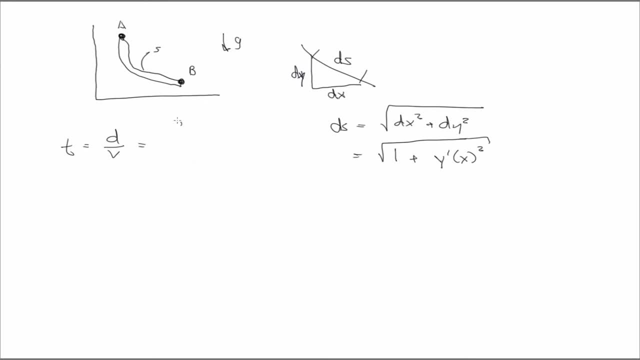 Okay, So then, mathematically, along our path, that'd be from point y1 to y2.. dS is the total path length over the velocity. That's equal to y1, y2, 1 plus y prime x squared over v. 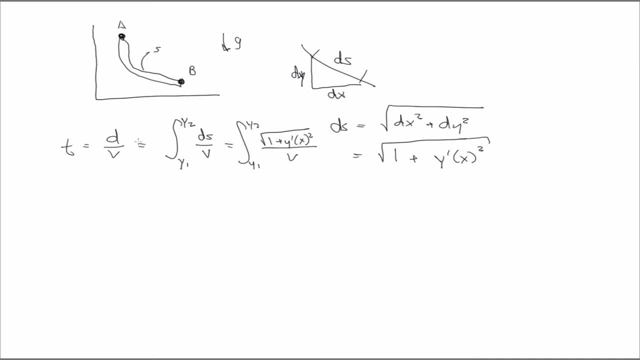 Right, And then just from statements of you know, we're just talking about a particle here, So we can say, just from conservation of energy of a particle that basically says the kinetic energy is equal to the potential energy, Well then that's 1 half mv squared equals to mg. 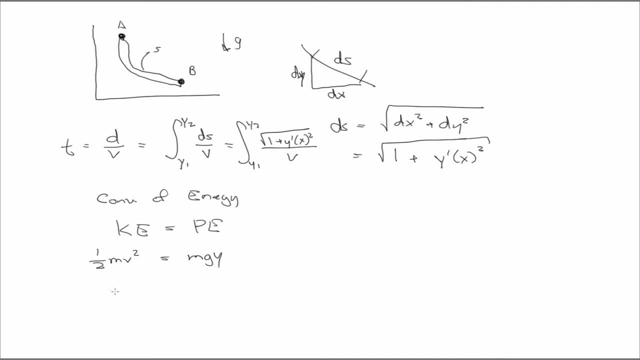 Y. Therefore v is equal to 2gy. So then if we plug that in back up there, we have finally that the time is y1, y2.. Oh, there should be a dx out here: 2gy minus dx. 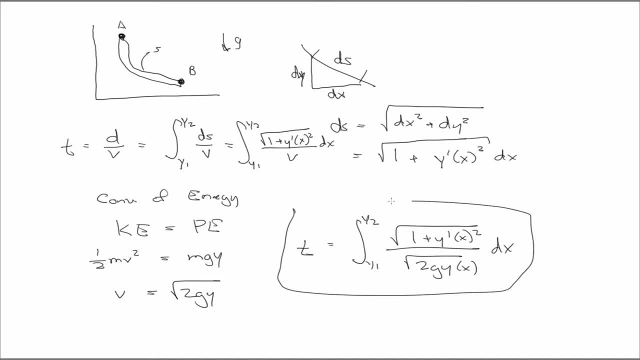 All right. So this is our model equation. And we want t to be a minimum, So we want to minimize t. So we're going to solve this equation for minimum t, Right? How do you do that? Hmm, That's how you minimize a function. 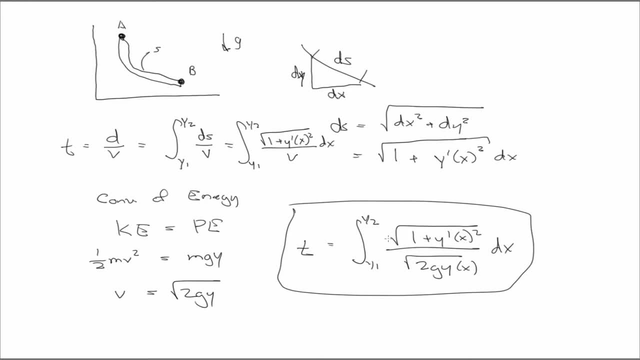 But what we have here is an integral or a functional, a function of a function, And so, yeah, you're right. And if it was a function, you'd take the derivative and you set it equal to 0 and you'd solve that, and the root of that equation would be the minimum. 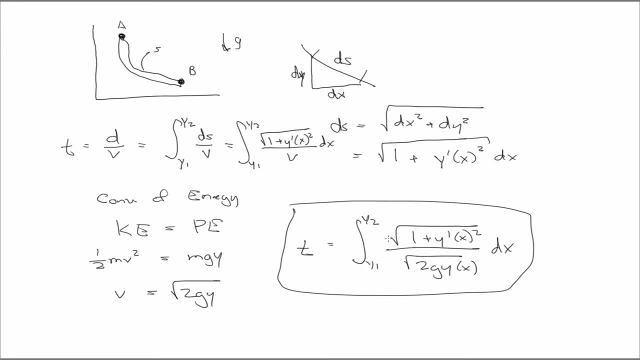 But it doesn't work for a functional. We have an integral here, So we want to minimize an integral. How do you do that? So it turns out- I mean, you probably don't know Who said variational theory- Okay. 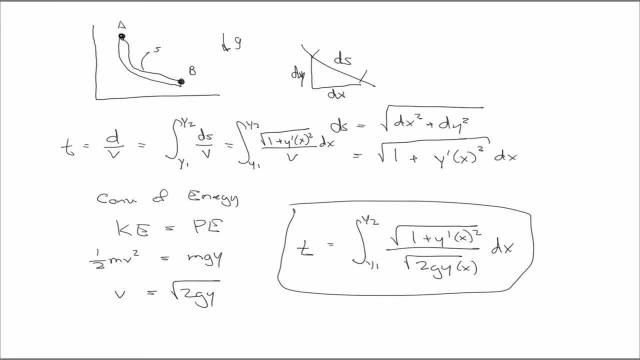 You've had a course in calculus of variations. Okay, So I mean, other than someone who's had a course in calculus of variations or seen it in some other course, you probably don't know how to do it, But this is exactly the whole realm of the calculus of variation. 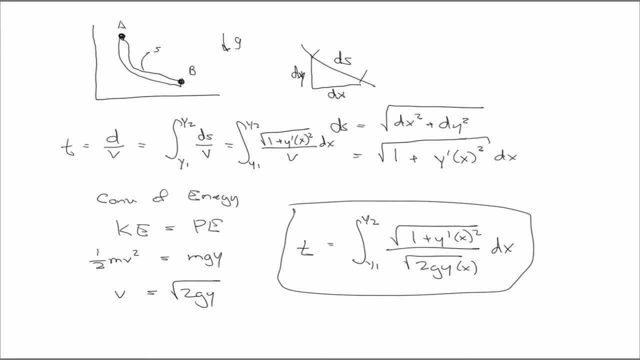 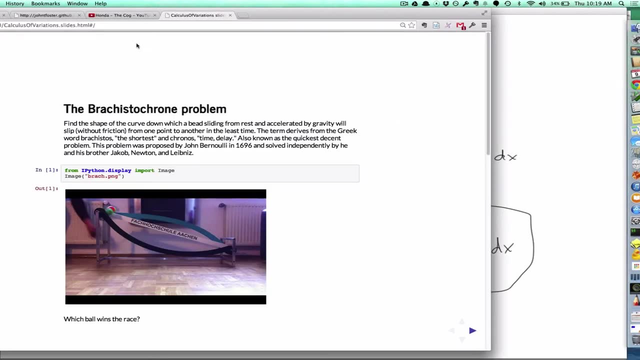 So we want to minimize, basically functionals or integrals. Okay, And so with that I'm going to switch back over And I'll make these notes available to you guys And the rest of this lecture I'm not going to do anymore. 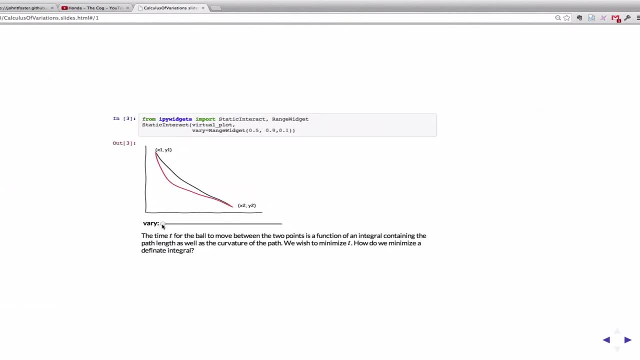 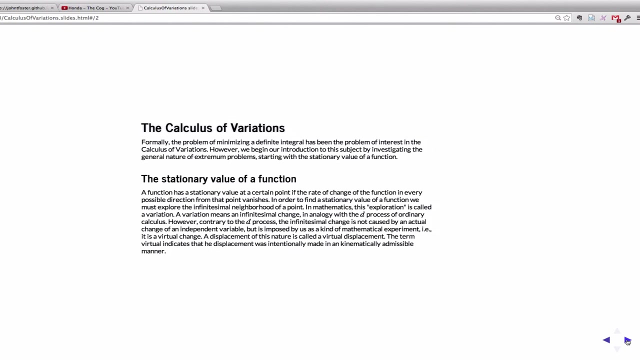 It'll just be the notes here And so yeah, basically, you know, just to kind of reiterate the problem, We're interested in exploring sort of all the paths, all of the possible paths between those two points. Okay, And this is where the calculus of variations comes from. 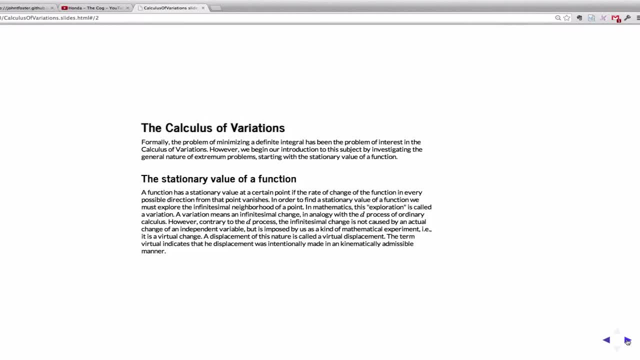 And the basic idea of the stationary value of a function. So- and I give some notes there, I'm going to kind of speed up because I want to get through this by the end of class. But all of you want to read what I have to say here. 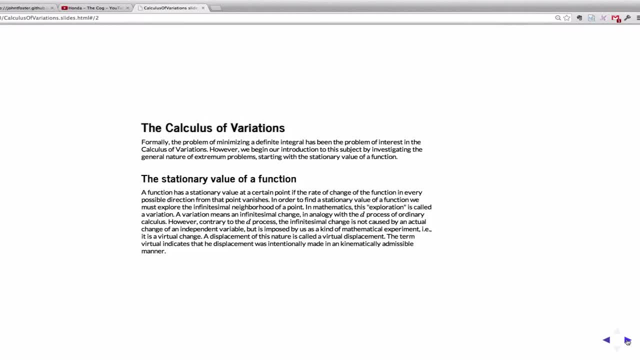 I'll make these notes available and you can say it. But basically, you know, the stationary value of a function is where the rate of change of any possible variation is zero. Okay, That would be a stationary value, And the easiest way or the easiest example I like to think of here is like a marble in a bowl. 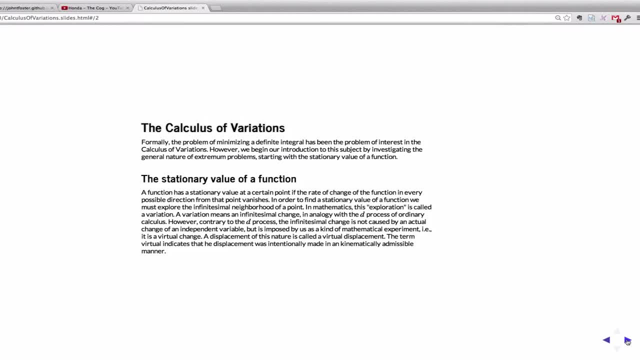 Right. It's obvious where the stationary value of that marble is Right: It's at the bottom of the bowl. Because if I at the very bottom of the bowl, if I move it in any direction, then the rate of change is basically zero. 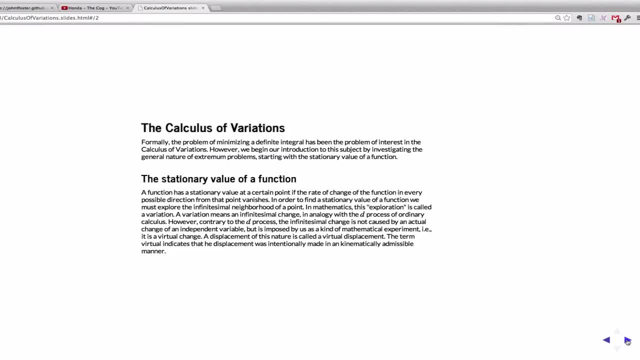 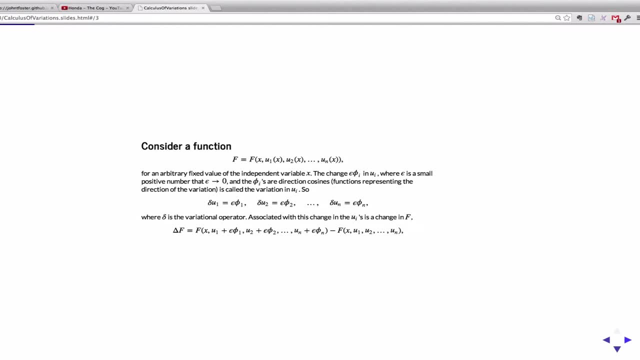 If I make any kind of infinitesimally small motion, And so if we consider a function that's in this case a function of X and some functions of X, So this is actually a functional right, Because U is a function of X. 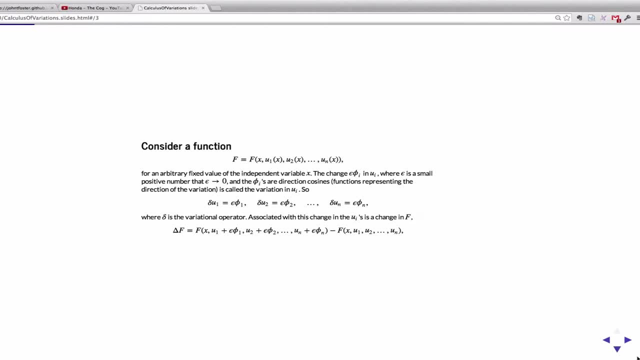 Okay, And we investigate A virtual change or a small change in U. Okay, And here I'm defining them with finite values. Where's my mouse? So, basically, I'm saying that the del U, or a small variation in U, is equal to some very small scalar that tends towards zero and some arbitrary direction phi. 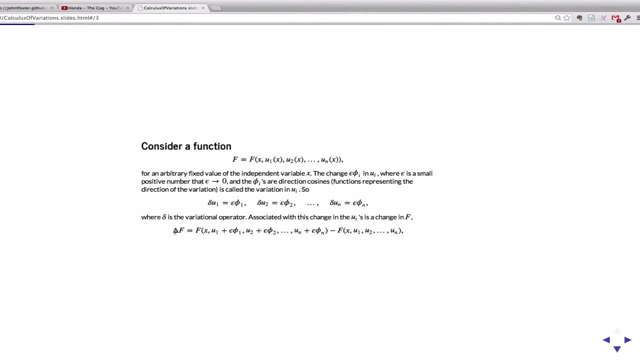 Some arbitrary direction, cosine Right. Well then, if I want to look at the change in the function, Then it's simply The function evaluated Plugging in, you know, with all these arbitrary chains in the U's minus the original function. 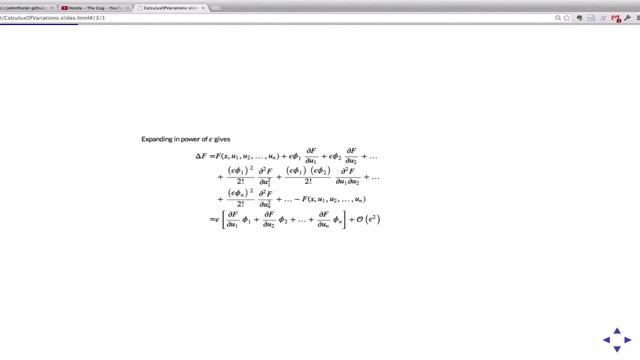 That's the change in the function. Okay, And so if we take that change in the function And we tailor, expand in powers of epsilon, Okay, Then eventually we arrive at this last equation And of course Epsilon Is something that tends towards zero. 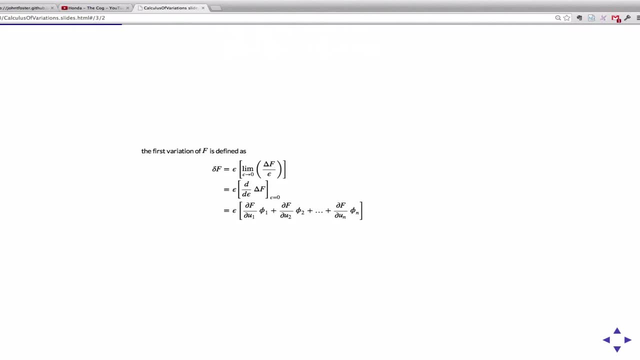 Right, So we can say that the first variation of F Is The limit of this. The change in F over E is, Or over epsilon, as epsilon goes to zero, And therefore, From what we just derived, You can see that you have. 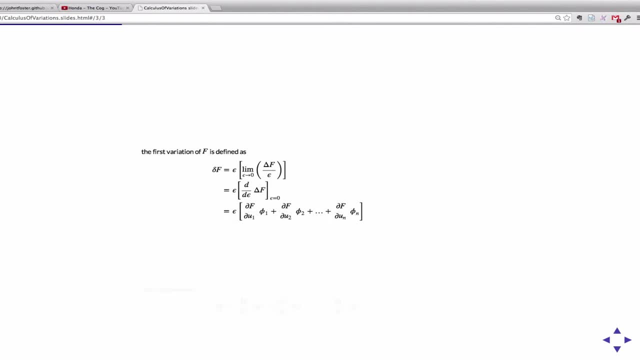 This guy Okay, This last equation Okay, But The Yeah, I think in the next slide I'll Yeah, So. So finally we have that the first variation of F Is equal to this, And if you compare that with the total differential of F, 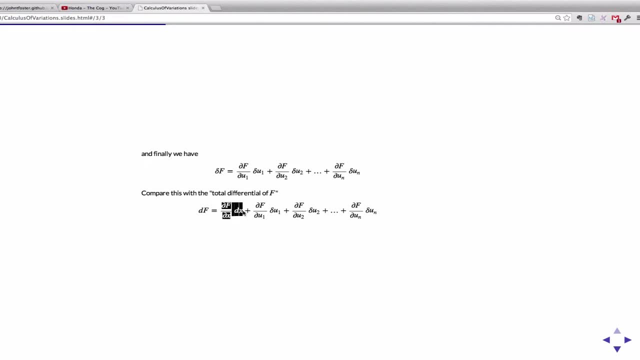 You have With the total differential of F, You have this first term, That's a function of Of X itself, And so These variations are performed In an instant in time, Or Yeah, I mean just With Holding time fixed. 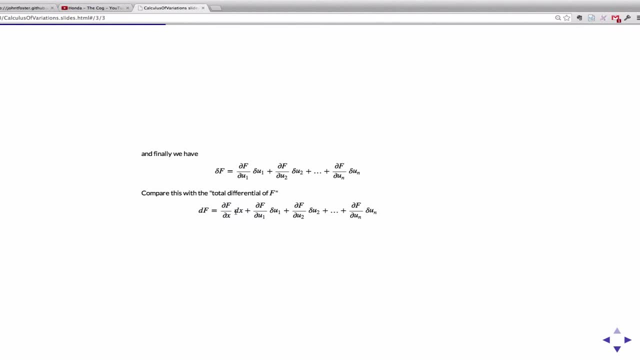 Okay, And performing these little variations, And so that's what makes them different Than a, Than a kind of standard. So then, This is more I'm. I'm trying to go fast here, I want to get finished, But 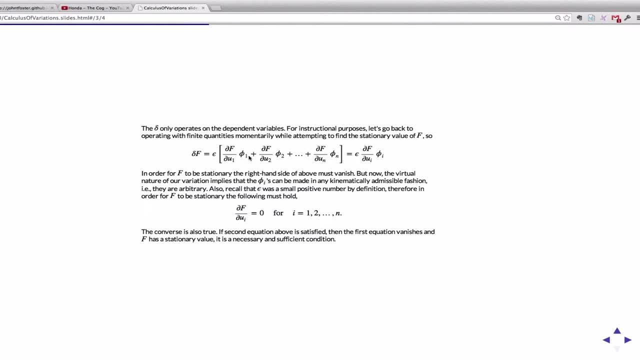 There's more kind of information about what I'm I mean here And we say that these, These direction cosines Are, Are arbitrary. So in order for F To be stationary Right, Then This The The right hand side. 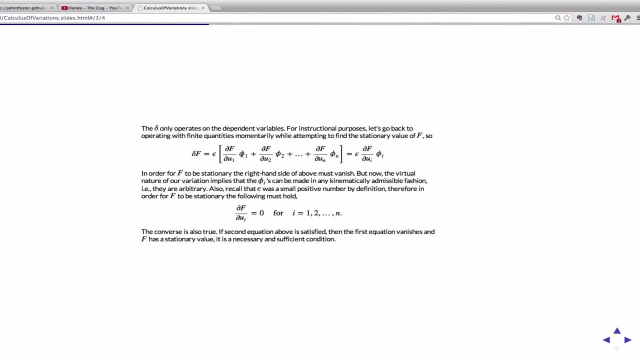 Must vanish. And if These Direction cosines Are arbitrary, Meaning they could be anything Right Because of the way we defined them at the very beginning, Then for that to be true, For For This to have a stationary value, 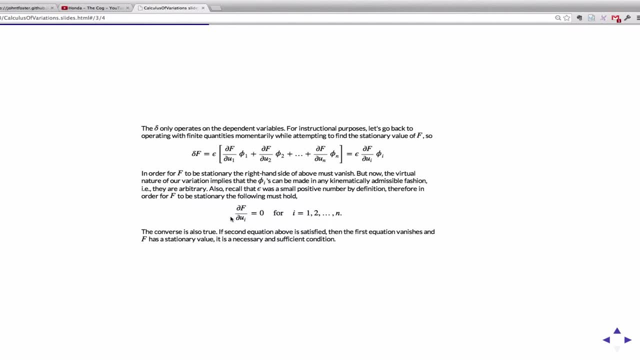 Then this statement must hold: Okay, So these are just some general notes on the calculus of variations And this Del Operator, It It is, You know, It's an operator Like the different Variations Operator Like the differential. 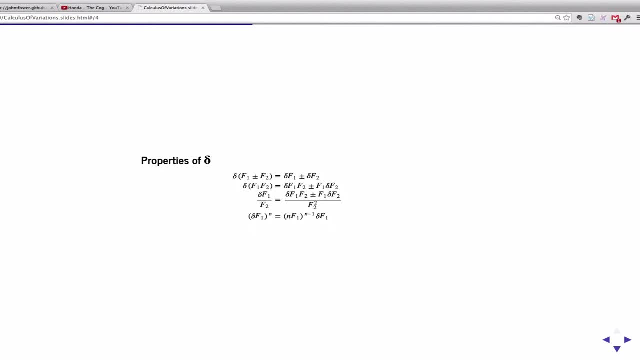 Operator, But not exactly the same, As I showed, But It's similar And Because of that It also has some similar properties In that It's, You know, It's commutative And you have a chain rule. 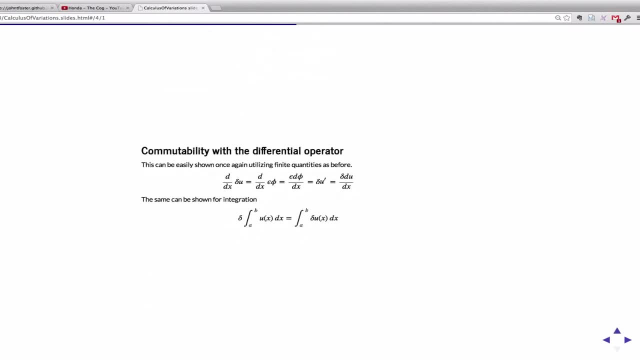 And a quotient rule And You know Product rule And all these things. Okay, It's also commutable With the differential Operator. So if you have D D X Of X, But you can show. 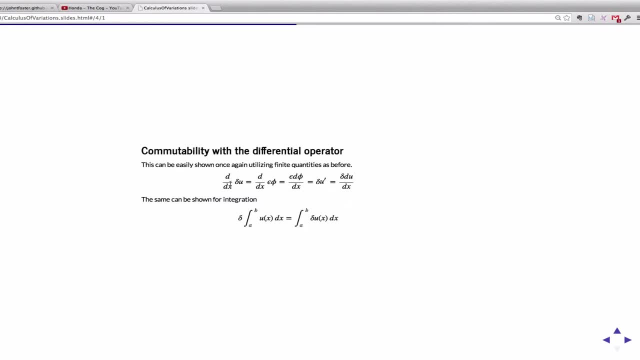 That it's commutative With the del. So you can, You can switch The order of operations With the, With the differential Operator, And we can also show The same For integration. And so Then There's also. 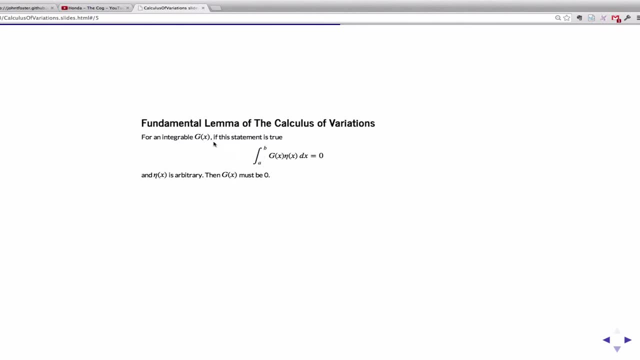 This thing Called The fundamental Lemma Of the calculus Of variations And it basically Just says That If you have, If you have An integral Function, If N Of X Is Arbitrary, 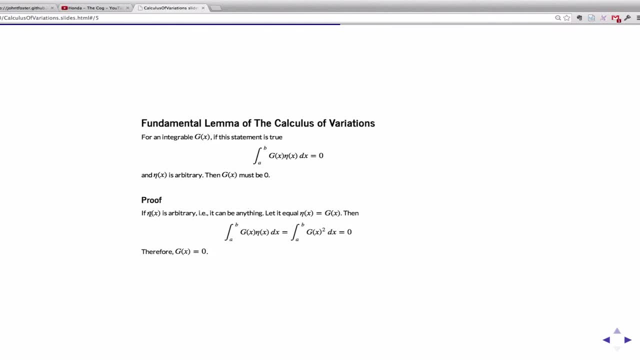 Then G Of X Must Be Zero, Okay, And We Can Show That By If N Of, If Eta That's Not N, Eta Is: 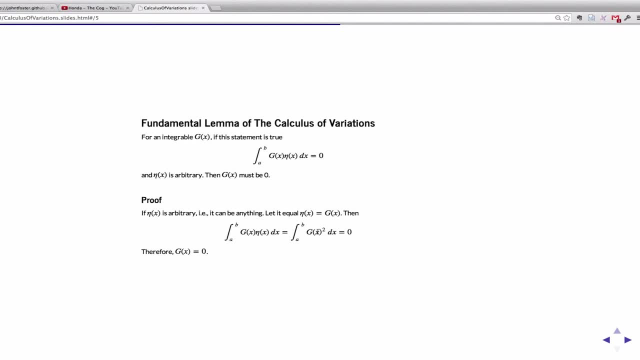 The Math. Math Is So Well Accepted, And It's All Rooted In The Calculus Of Variations, But So I Encourage You To Go. 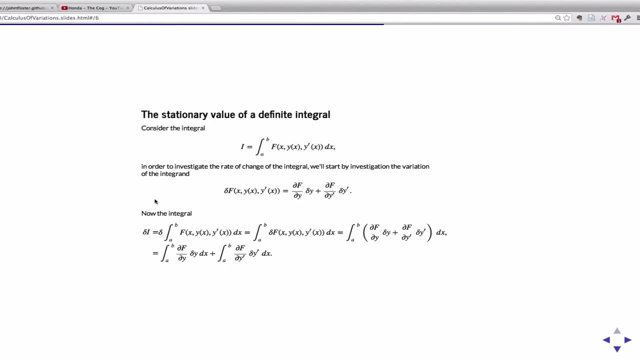 Look At These Notes In The Variational Operator To Investigate The Stationary Value Of A Definite Integral. I'm Basically Just Doing Some Mathematics. 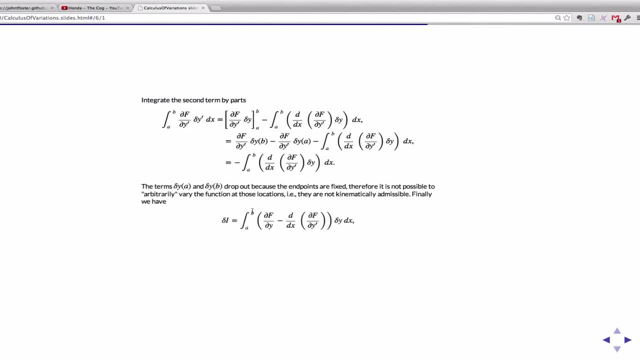 That Are Consistent With What I. The Way I've Defined The Del Y Is Arbitrary, Then What's Left For This To Be Stationary Is? 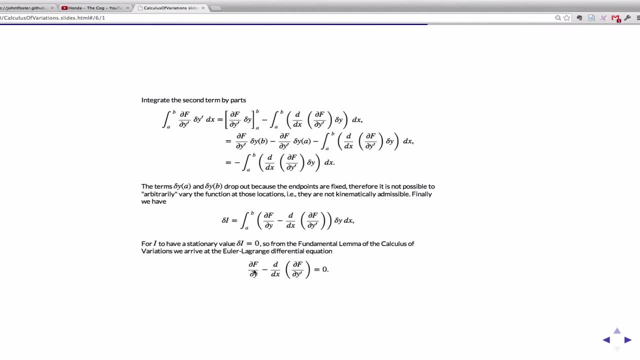 That What's Left Is. The Integrant Here Has To Be Equal To Zero And This Thing Right. So We Basically Just Plug In The Integrant. 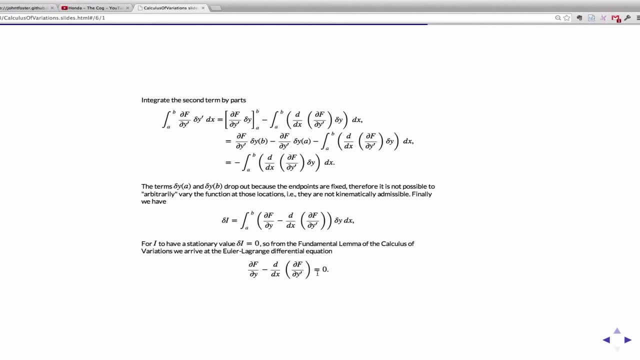 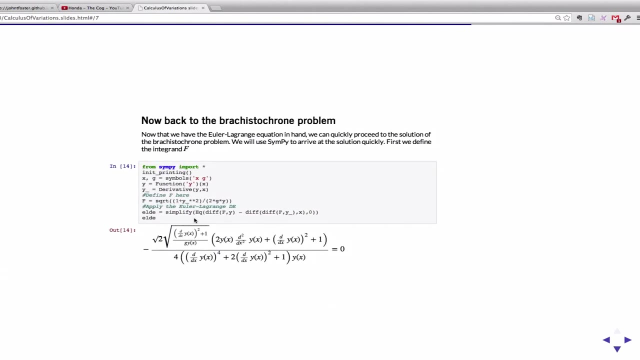 You Know, F Equals The Integrant Of The What We Derived Earlier, And You Apply The Machinery Of The Code Here, So I Actually Use 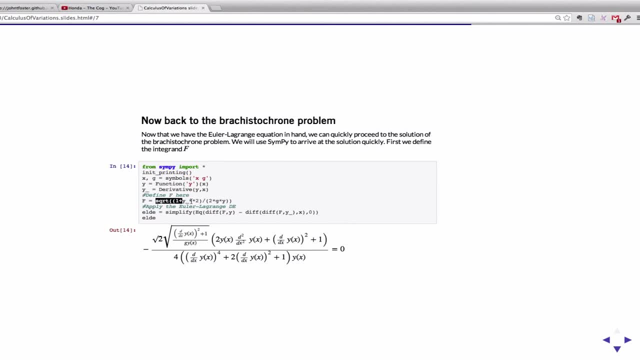 Some Senpai In Python Here, But Basically You Know I Define Our Function. The Function Is The Square Root Of One Plus Y. With Respect, 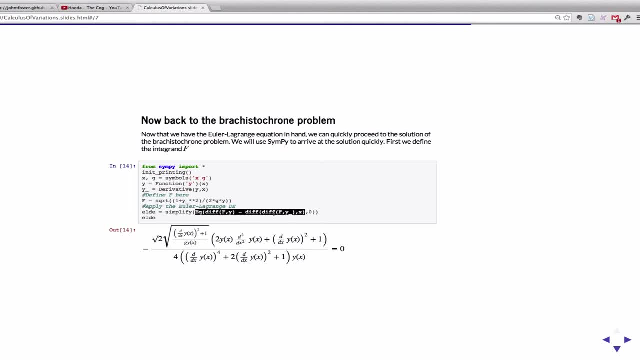 To Y, The Differential Function With Respect To Y And Then Again With Respect To X. Simplify It All, Set It Equal To Zero And 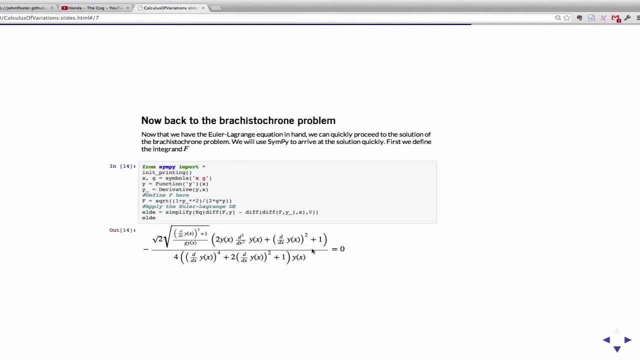 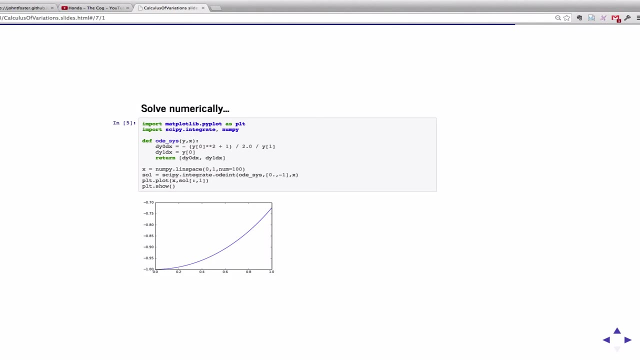 You Get The Differential Equation. I Know It's Hard For You Guys To See That's D Square D X. So This Thing Right Here Is. 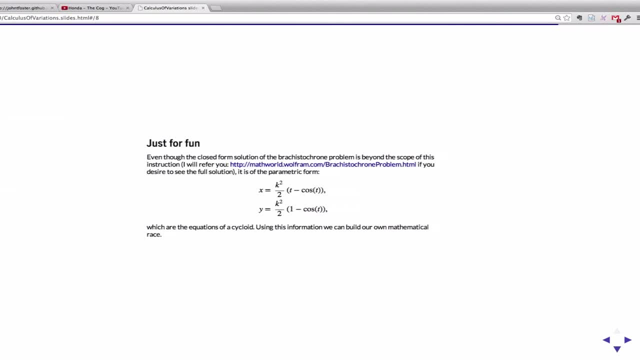 A Differential Equation That We Need. So Turns Out, You Can Here Here. I Just Solved It Numerically. I Just Solved That Differential Equation.